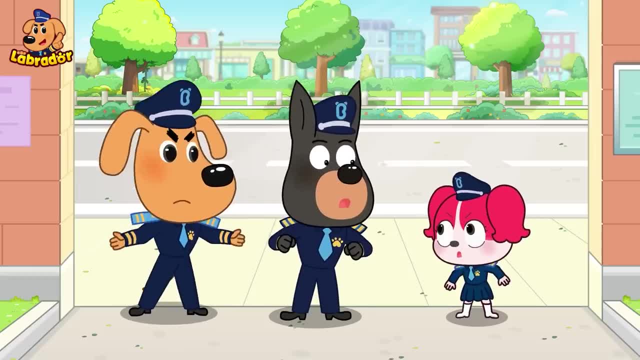 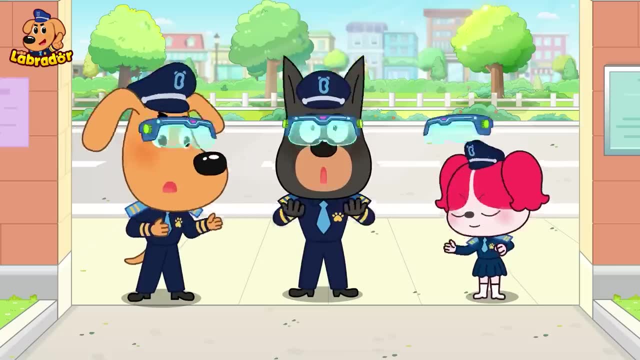 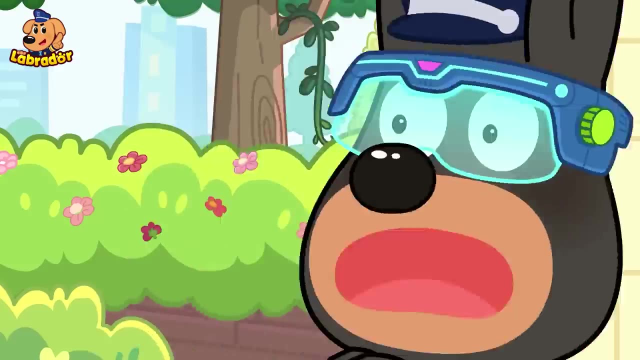 There might be bugs, Viruses, going around. Papillon, check it out. Okay, Wear my super goggles, They can help you see germs around you. Cool Wow, Sheriff Labrador, your nose is so big Toby adjust them from here. 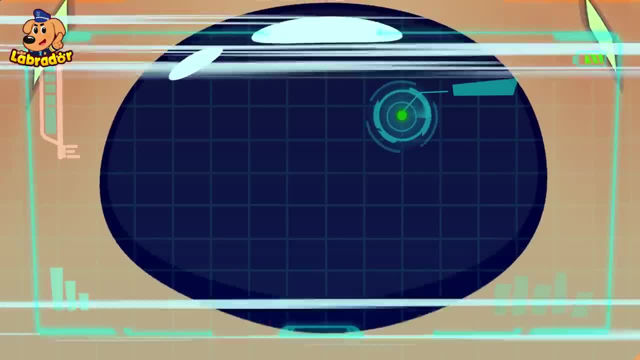 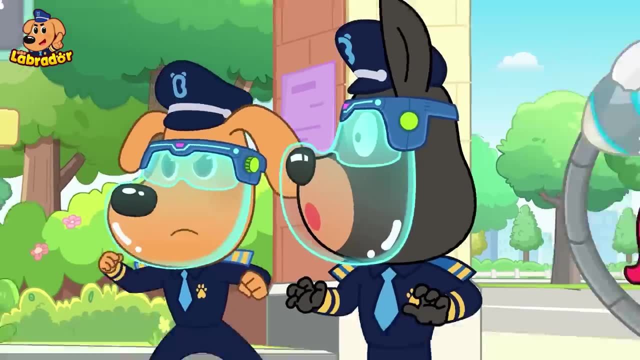 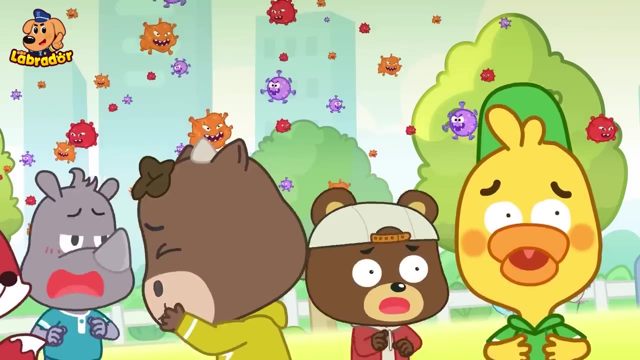 Here. Ah, So many viruses. Get the kids out of here. They need to go to the hospital, Got it? Huh, Kids, there are many viruses here. You have to leave this place right now. This way, Hurry up. 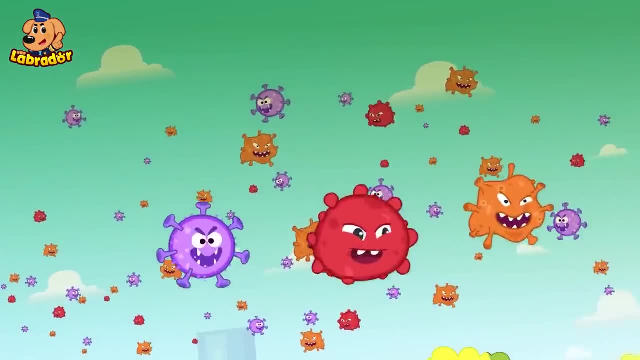 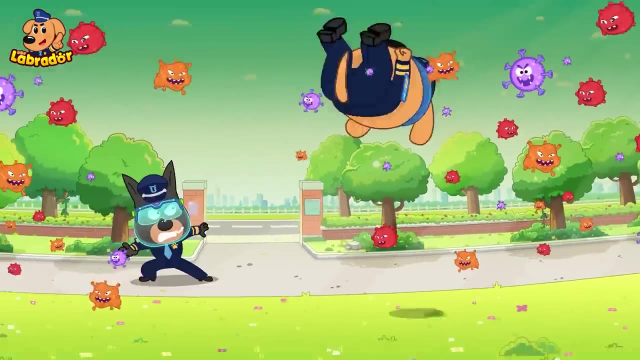 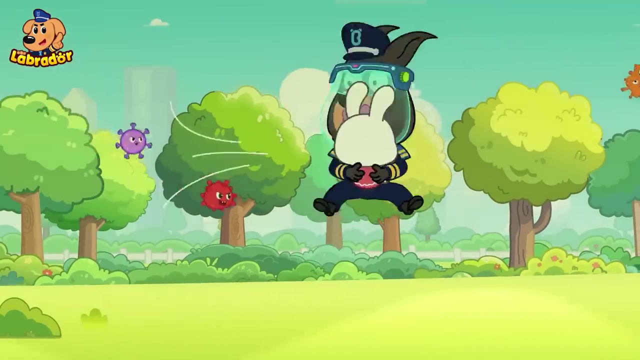 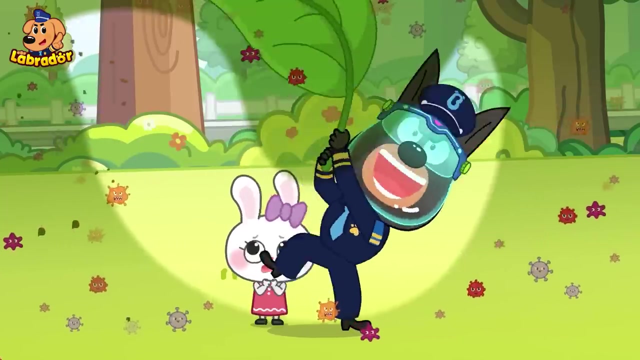 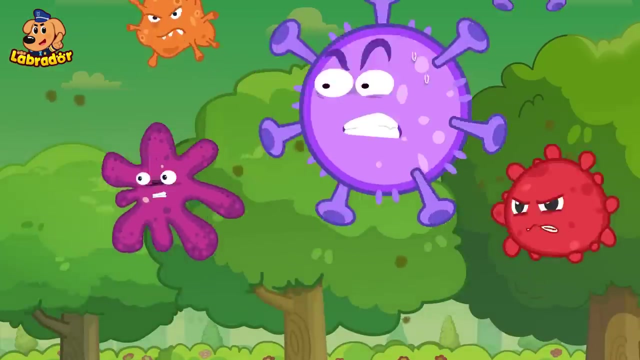 Achoo, Be careful, Be careful, Ah, Ah, Ah, Ah, Ah, Go away, Can't blow them away. That's it. Take this. viruses, Watch me. Ah Huh, They're coming back. 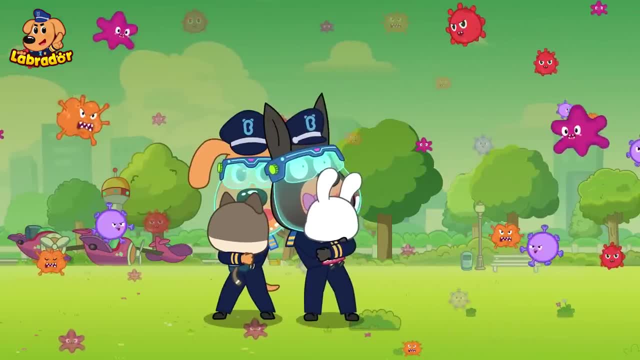 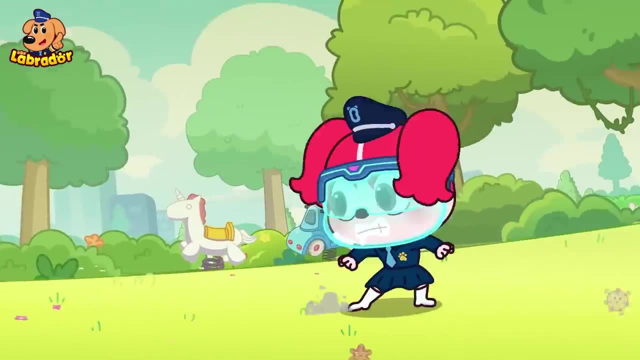 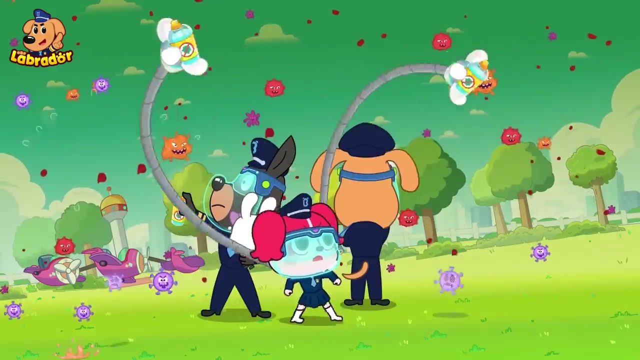 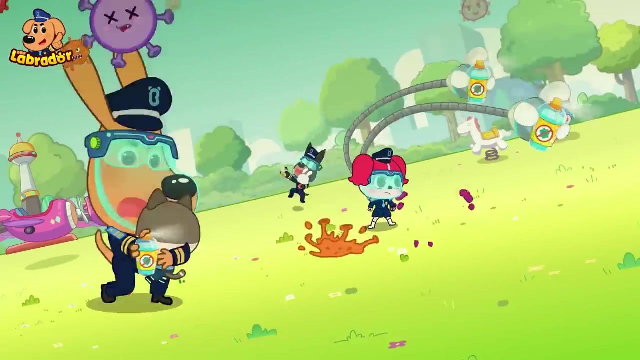 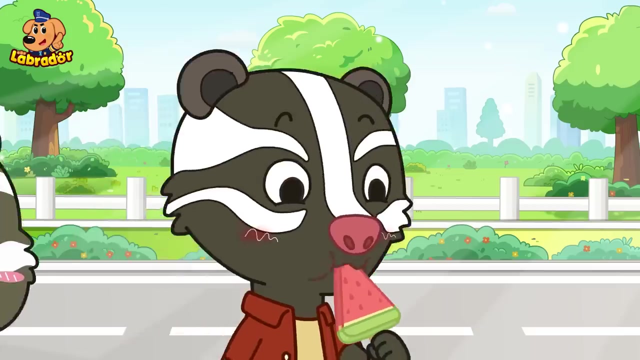 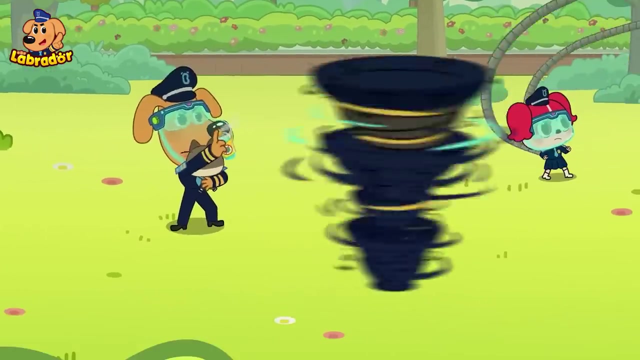 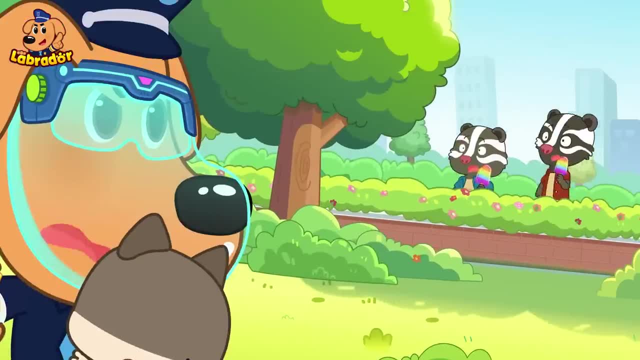 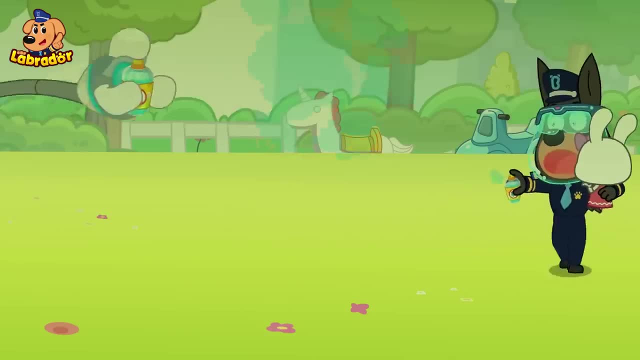 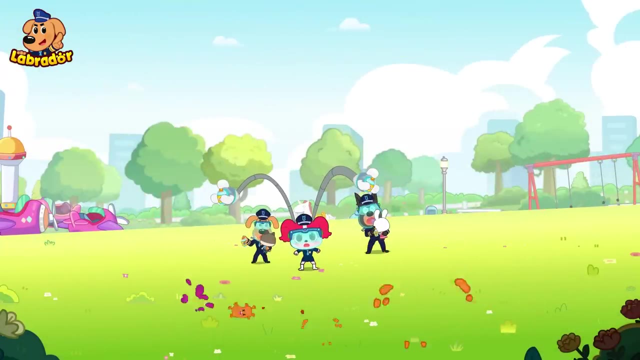 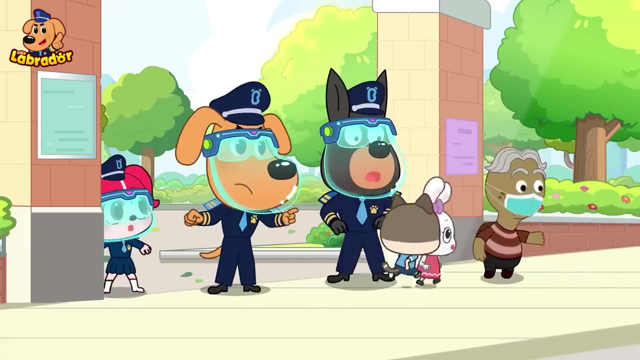 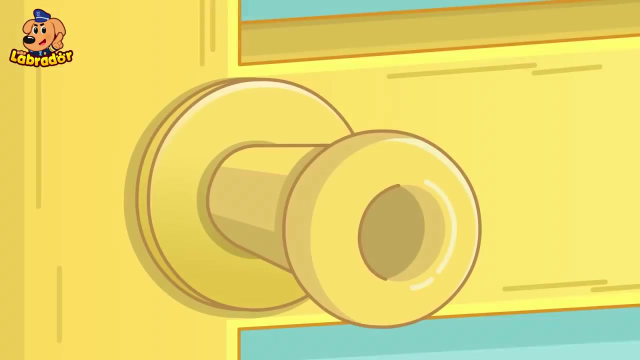 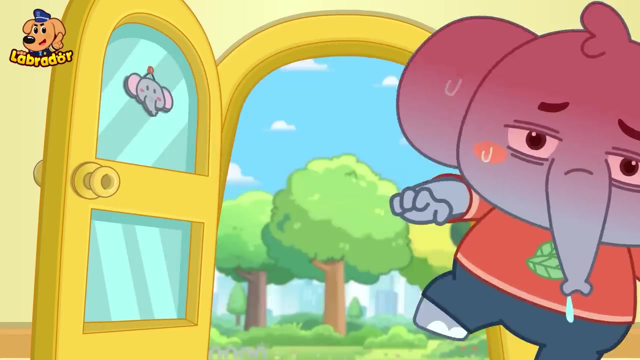 They look so funny. There are many viruses here. Run, Watch me. You guys go see a doctor. Follow the viruses to check out where they're from. Mommy, I'm not feeling well. I think I'm sick, Mommy.